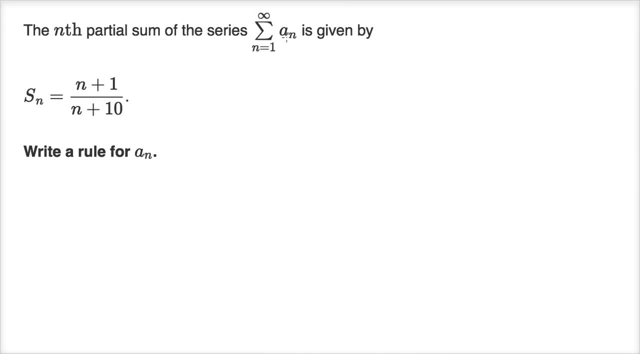 Partial sum of the series. we're going from one to infinity. summing it up of a sub n is given by and they tell us the formula for the sum of the first n terms and they say: write a rule for what the actual nth term is going to be. 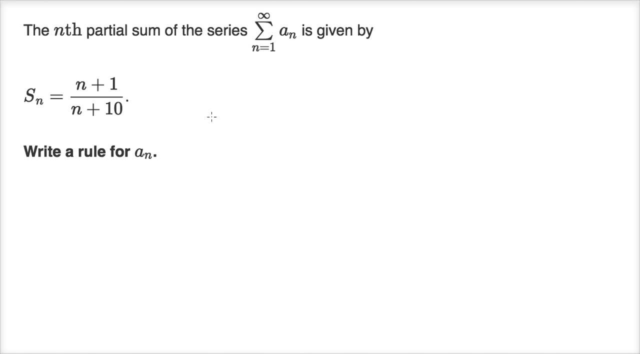 Now, to help us with this, let me just create a little visualization here. So if I have a sub one plus a sub two plus a sub three, a sub three, and I keep adding all the way to a sub n minus one plus a sub n. 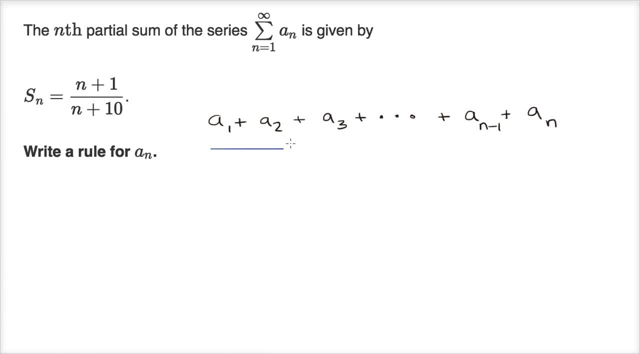 this whole thing, this whole thing that I just wrote out, that is s sub n. This whole thing is s, let me, this whole thing is s sub n, which is equal to n plus one over n plus 10.. Now, if I want to figure out a sub n, 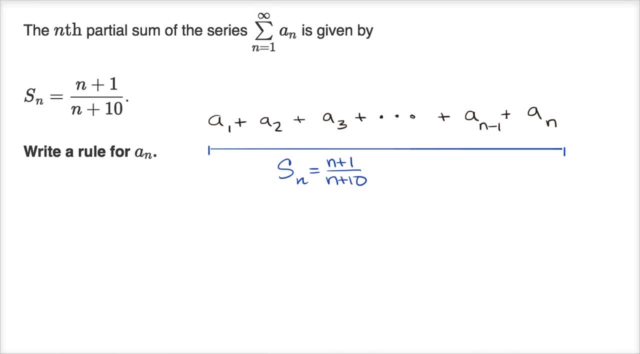 which is the goal of this exercise. well, I could subtract out the sum of the first n minus one terms. So I could subtract out this: So that is s, that is, s sub n minus one, and what would that be equal to? 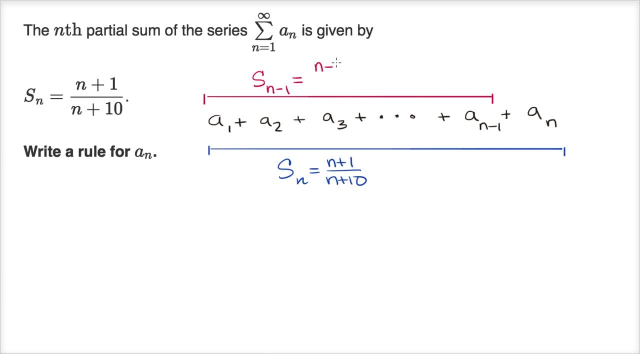 Well, wherever we see an n, we'd replace it with an n minus one, so it'd be n minus one plus one over n minus one plus 10, which is equal to n over n minus one, So that would be n plus nine. 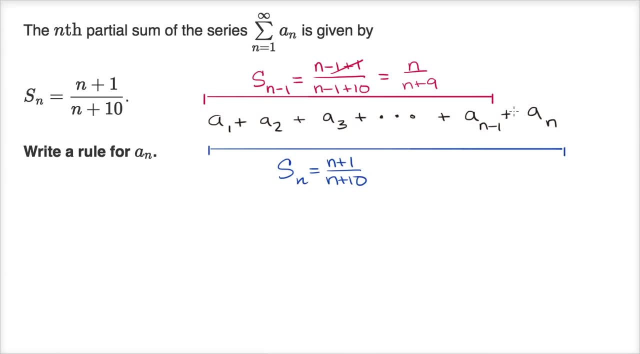 So if you subtract the red stuff from the blue stuff, all you're going to be left with is the thing that we want to solve, for You're going to be left with a sub n, So we could write down: a sub n is equal to s sub n. 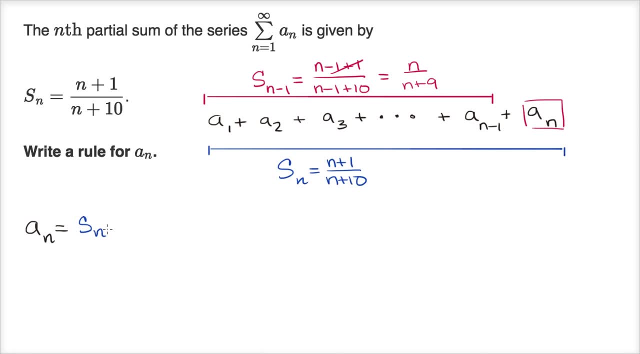 is equal to s sub n minus s sub n minus one, s sub n minus one. or we could write that is equal to this stuff. so this is the n plus one, n plus 10 minus n over n plus nine, And this by itself. this is a rule for a sub n. 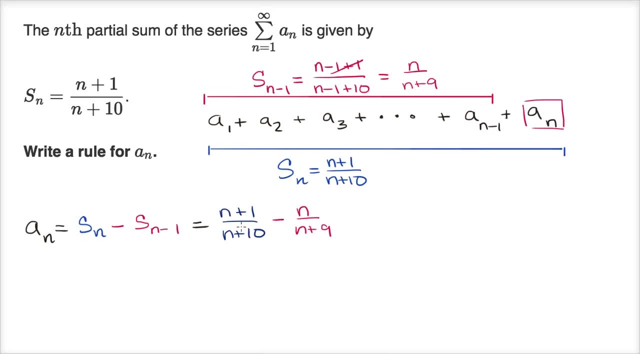 but we could combine these terms, add these two fractions together and this is actually going to be the case for n greater than one, For n equals one s sub one is going to be: well, you can, just a sub one is going to be equal to s sub one.